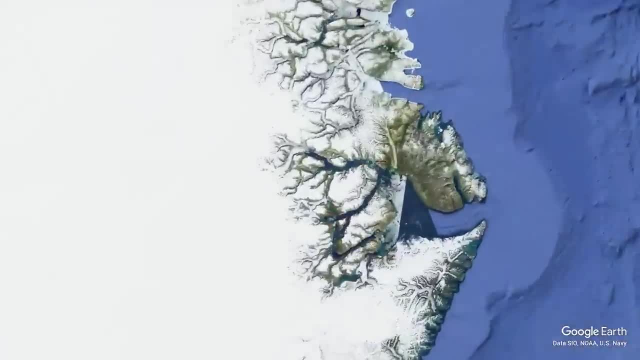 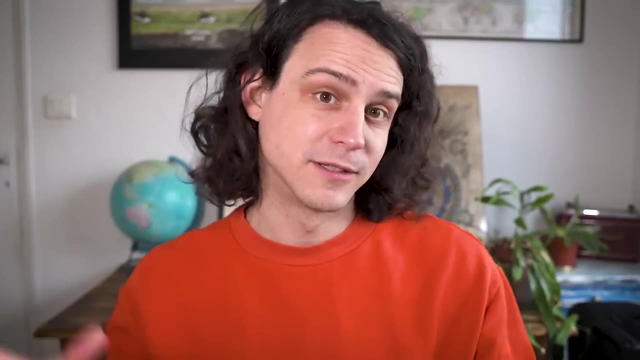 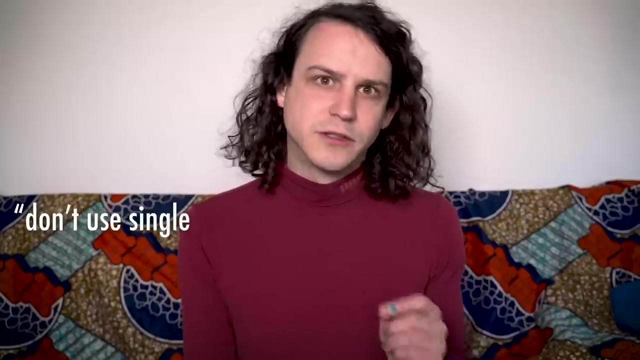 each one only captures what's happening in one specific place, So you can't rely on one single source of this data. You have to combine multiple sources to get an accurate result, And remember that because it's going to be important later. Don't use single source of data for prehistoric. 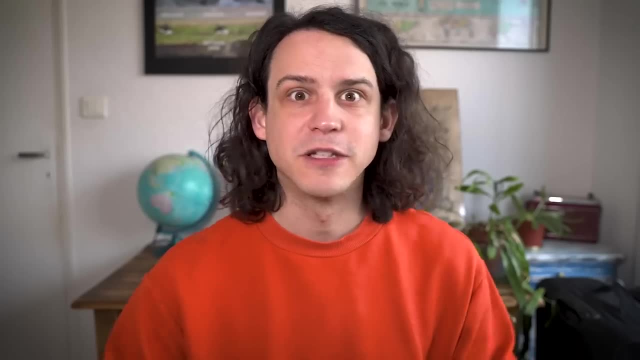 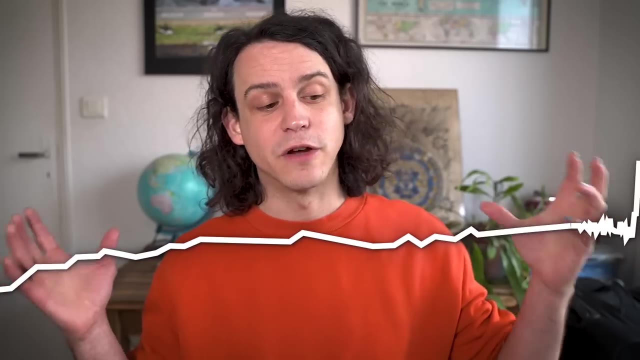 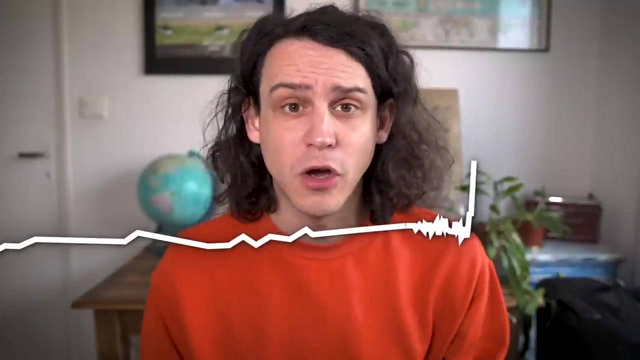 temperatures Noted. By using detailed measurements from all over the world carefully combined using the latest techniques, you end up with this record of global temperature change for the last 10,000 years, highlighting just how extreme modern global warming is and how much we're messing up our planet. 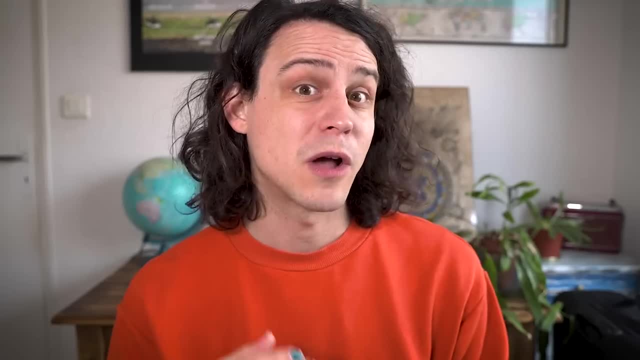 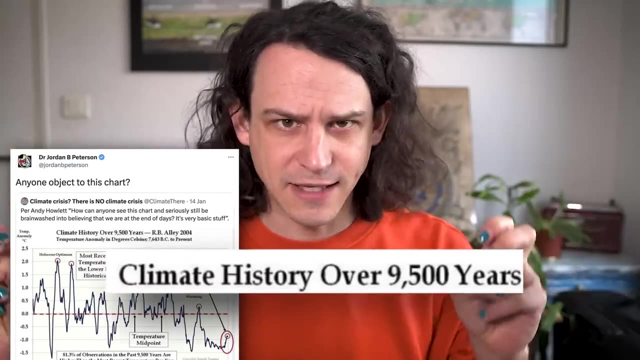 our home. And speaking of messing things up, let's talk about a tweet from Jordan Peterson which appears to show Climate history over 9,500 years Straight off the bat. this graph is going to look weird because, well, because it doesn't look. 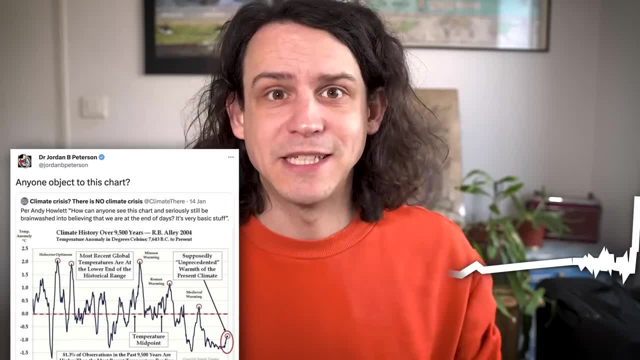 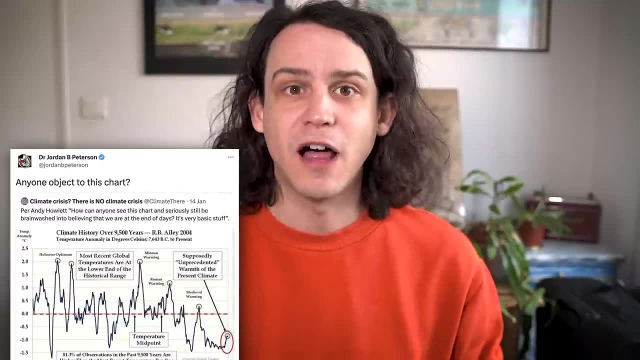 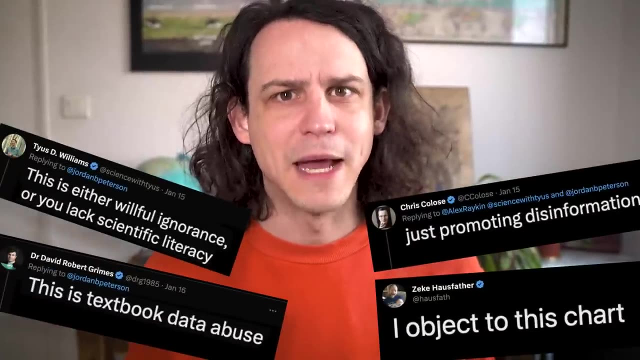 anything like the graph I just showed you. Jordan Peterson asks anyone object to this graph, Which sounds like a rhetorical question, but it has a very real answer, which is that, yes, I and many other climate scientists object to this graph for many, many reasons. 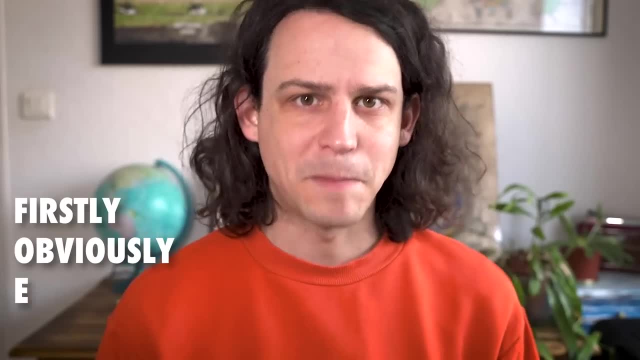 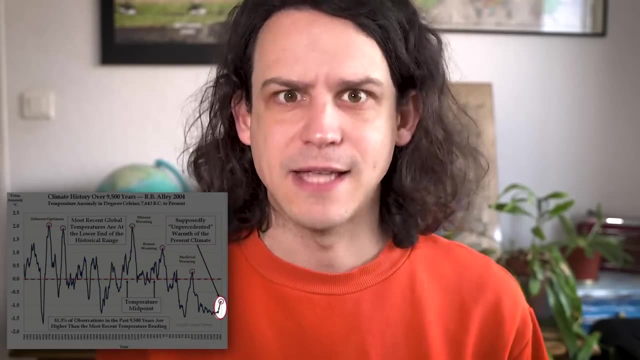 Firstly, most obviously and, let's be honest, most embarrassingly, the graph ends in 1885.. They circle this little bump at the end as if to say: look how tiny recent global warming is. but then they have actually left out. 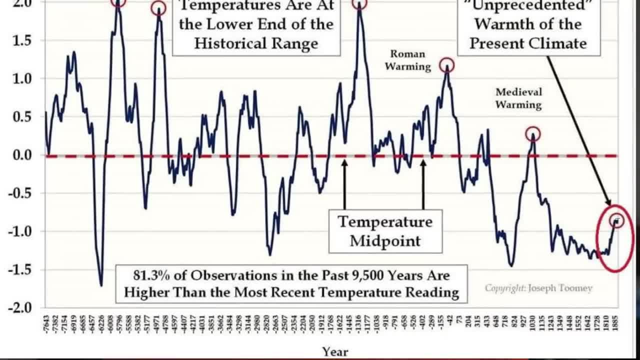 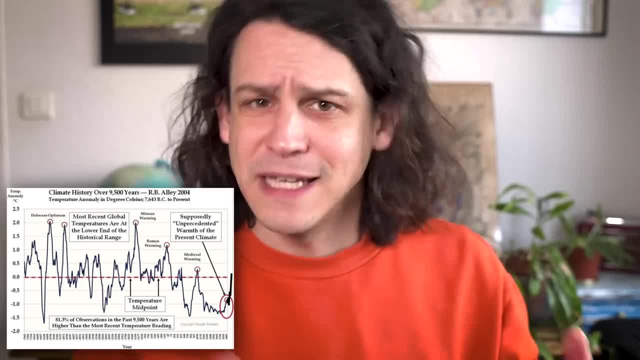 all of the recent global warming. For context, this is what this graph would look like if it ended today. But speaking of the end of the graph, this data set that this graph is made from actually ended in 1855.. 1855.. 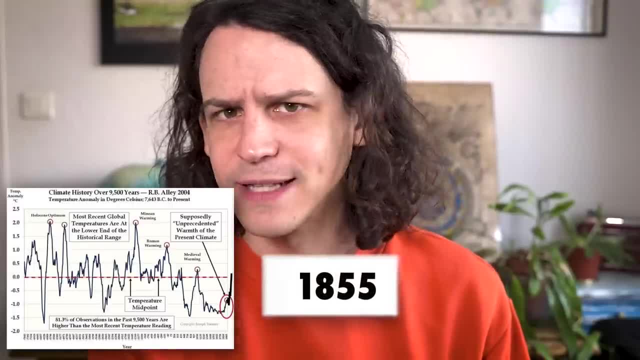 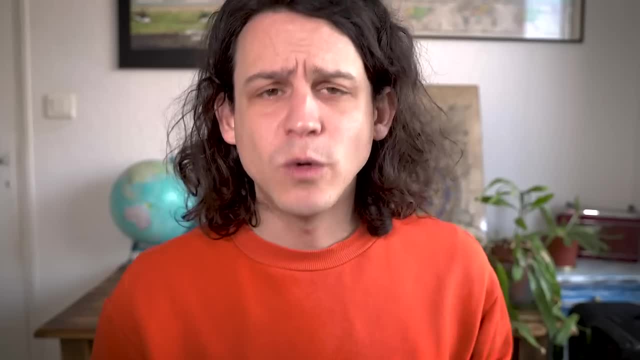 1855.. So either they're lying on the axis or they've just made a typo, and I don't actually know which is a bigger fail. But even once you take into account that this graph leaves off all of modern global warming, you can see that 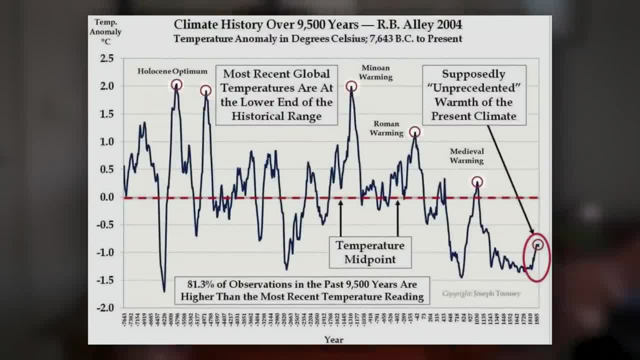 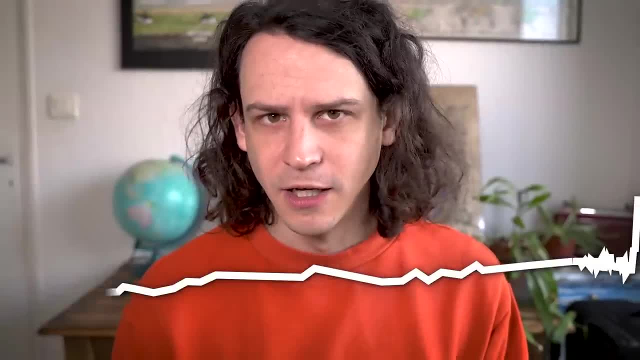 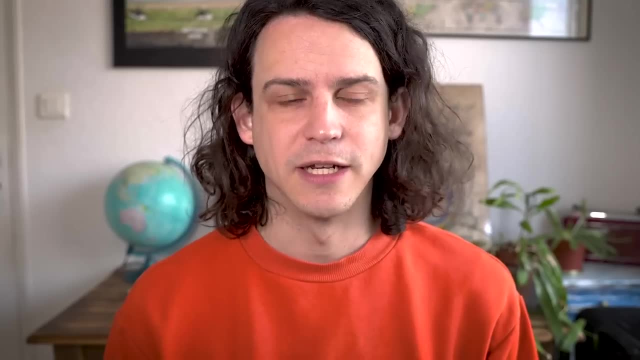 something's not quite right. What's with all these spikes that are ominously circled in Microsoft Paint? Why weren't they in the data set that I showed you earlier? Well, this graph from Jordan Peterson is taken from a single core of ice from a single location in Greenland. And remember when I said to you earlier: 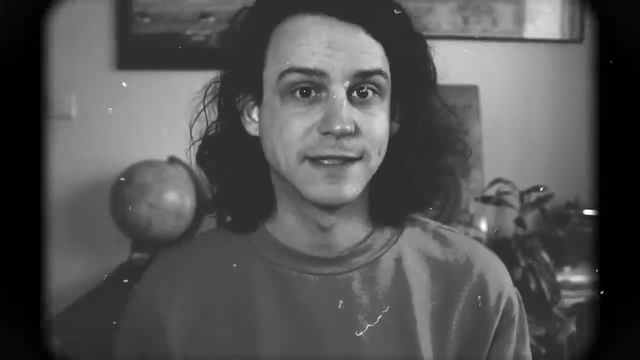 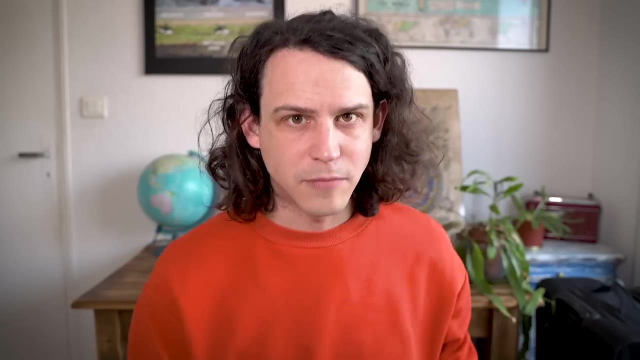 so you can't rely on one single source of this data. These sharp peaks and valleys don't mean anything when you're looking at a single ice core, because there's just so much scientific uncertainty. In fact, the scientists who are responsible for putting together the temperature record over the past 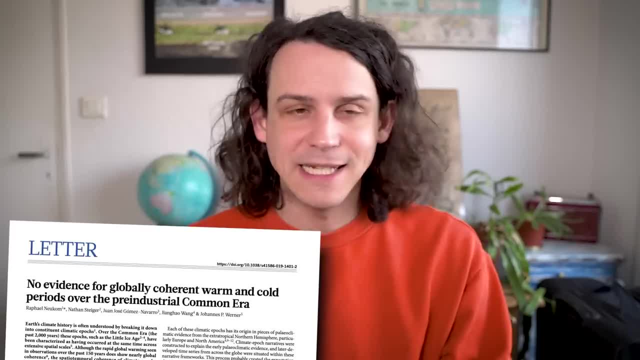 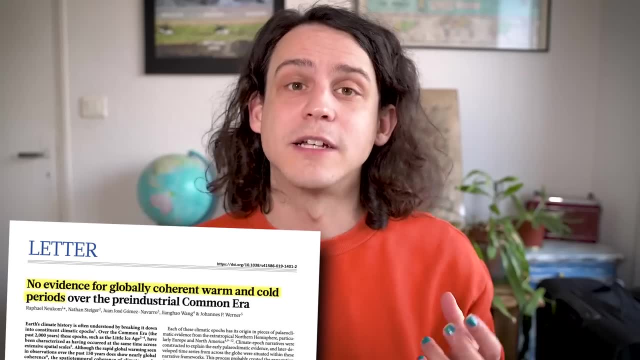 thousands of years put out evidence that the temperature record of the past thousands of years put out a paper explicitly saying that there's no evidence for sharp rises or decreases in temperature when you look at Earth as a whole. Well, apart from the temperature, 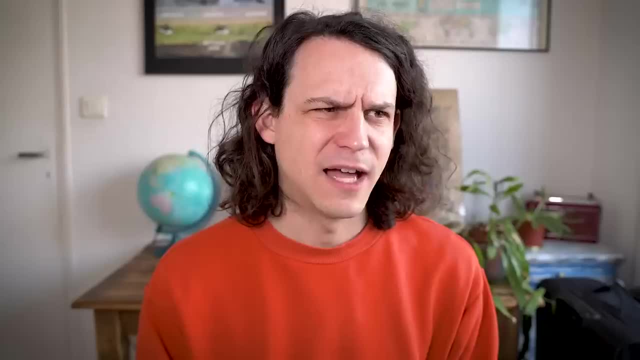 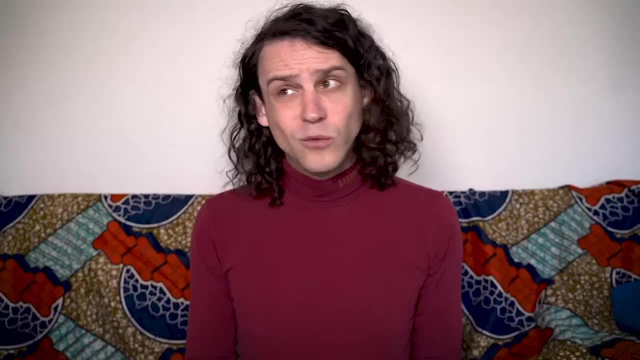 spike that we've been causing for the past century or so? Yeah, apart from that one, Okay. but why should I trust you and the other climate scientists who pointed these things out? Yeah, why should I trust you and all the other climate scientists? 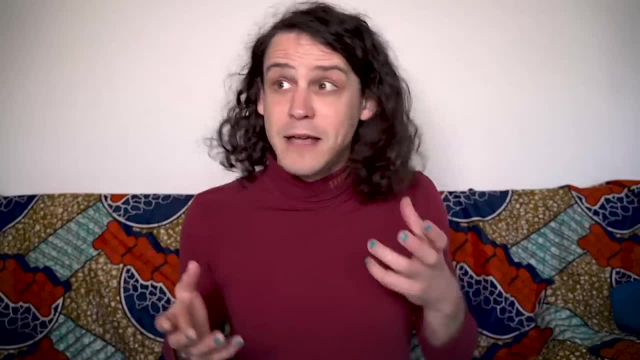 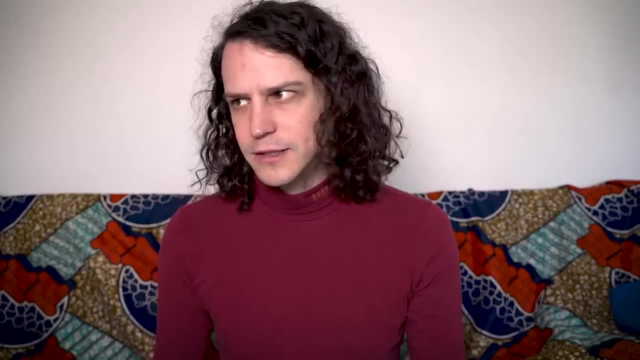 who pointed these things out? What about the climate scientists who actually came up with this data? So glad you asked. It's literally on the script that you gave me that I have to ask. Richard Alley, the scientist whose name is on the graph, had this to say: 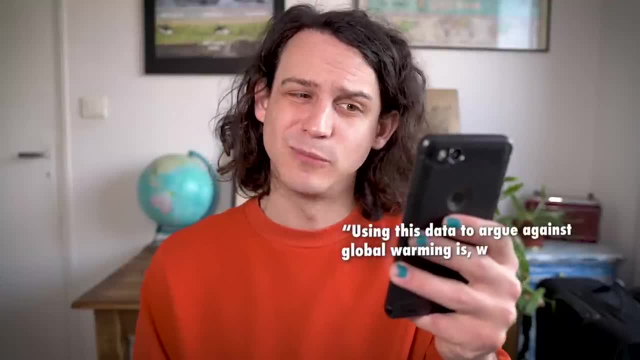 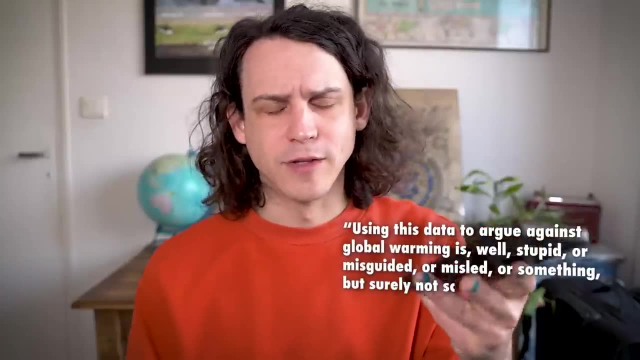 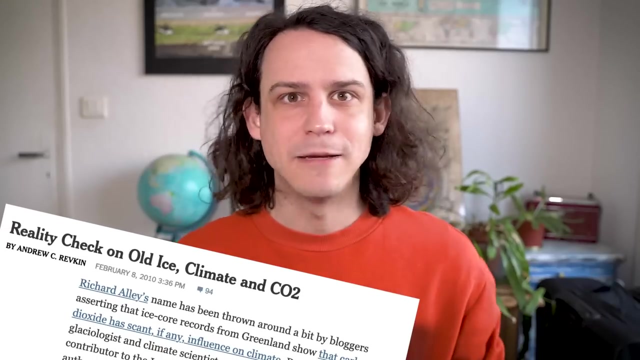 Using this data to argue against global warming is well, stupid or misguided or misled or something, but surely not scientifically sensible. So not exactly a glowing endorsement. In fact, Richard Alley said this way back in 2010,, when he said: 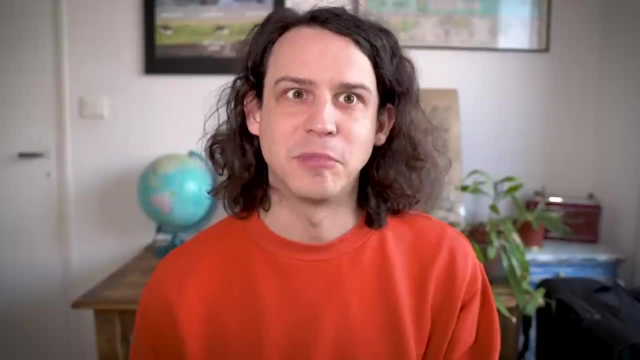 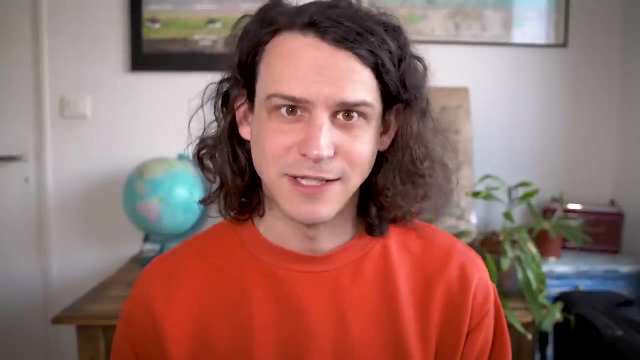 because- shock horror. this isn't the first time people have misguidedly misused his data set to try to mislead people about global warming. Richard Alley has referred to this misinformation as a climate zombie that just won't die. So to sum up this graph that 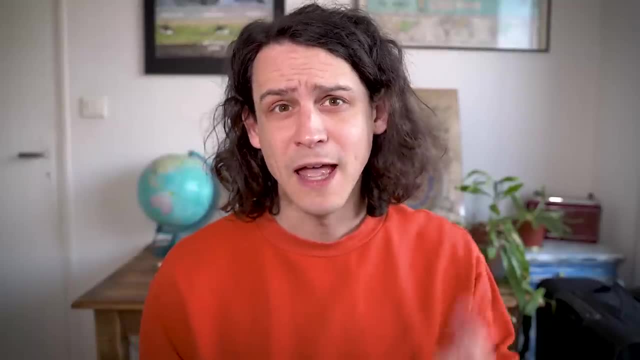 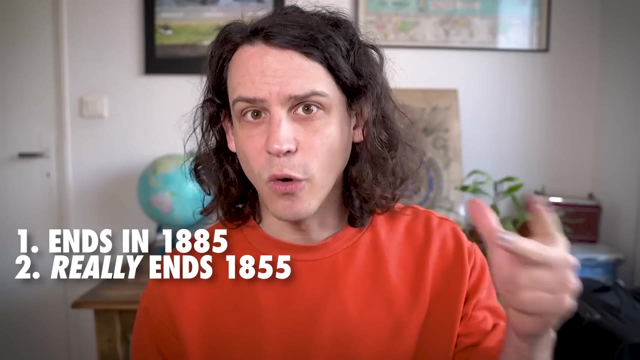 claims to disprove the significance of modern global warming ends before modern global warming starts lies about where it ends, and it is based on a single core of ice, and so it has error bars far too high, and so it has error bars far too high, and so it has error bars. 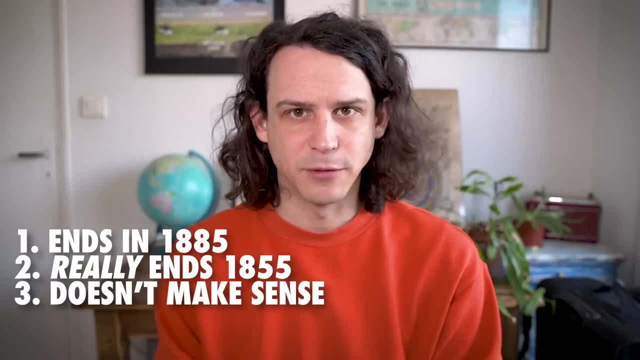 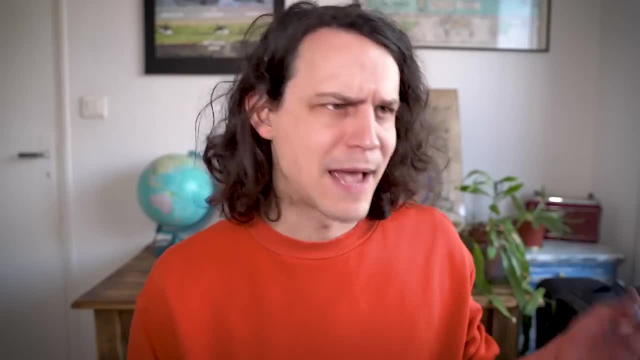 far too big for anyone to draw any significant conclusions from it. So wait, I'm getting mixed messages. Do you like the tweet or not? You mean this tweet which asks whether anyone has any objections and then was met with objections from: basically, 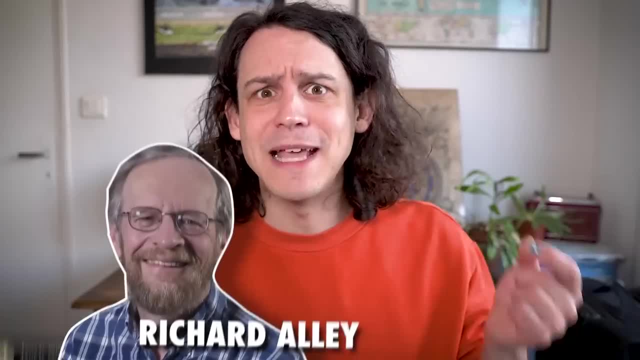 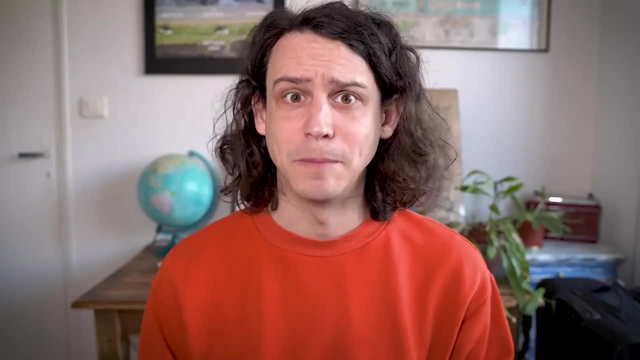 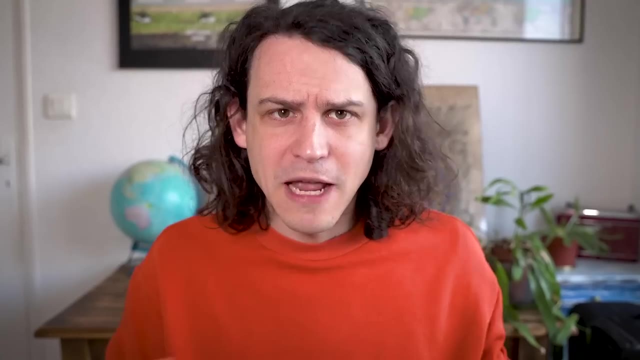 all climate scientists, including the one whose name is on the graph. Yeah, I'm not a fan- And this is what I really want to talk about- about Jordan Peterson's approach. He acts as if he's just asking questions. just curious, perfectly reasonable, academic. 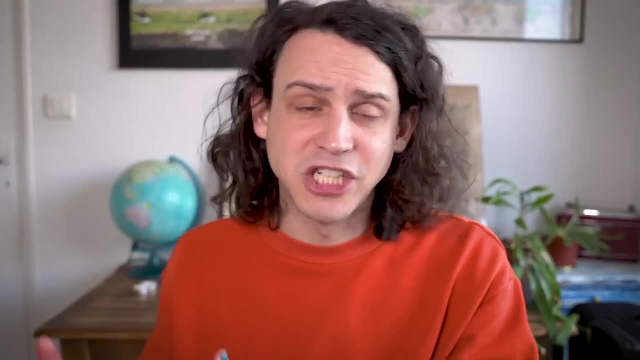 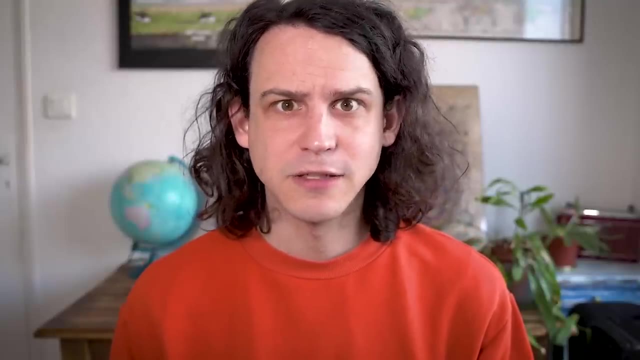 But if that's his approach, why doesn't he do the most basic fact-checking first? And if he had a little humility and could accept that he's not an expert in climate science, he could just call a climate scientist up. I mean, hell, he could start with the climate. 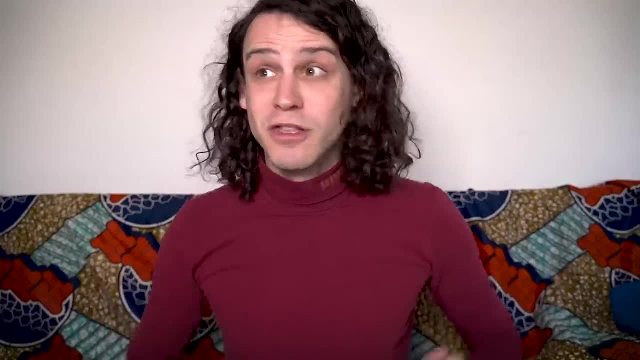 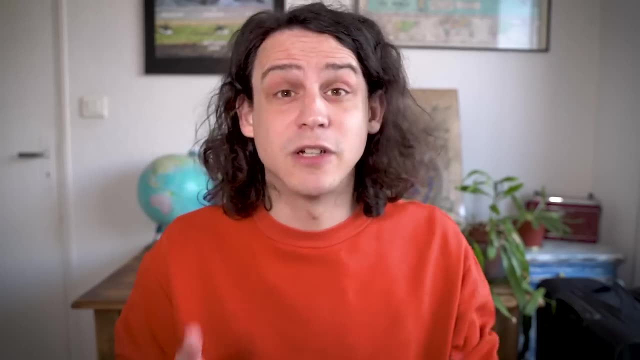 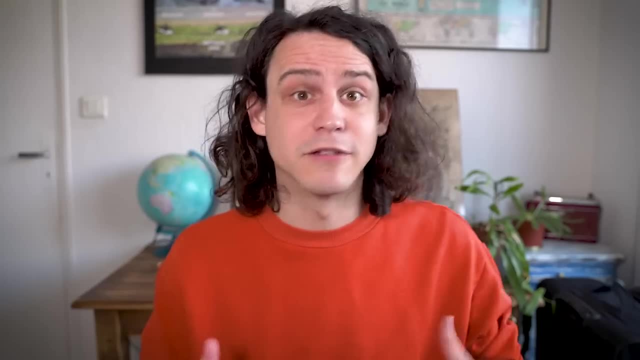 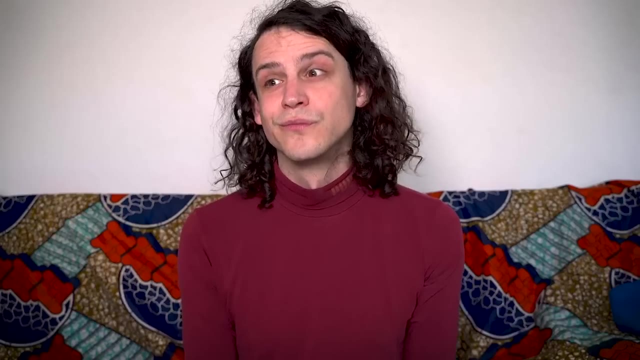 I don't know, I don't know, I don't know. Well then, he's had plenty of time to see and read the responses of experts to his tweet. Why hasn't he taken down this misleading graph now Or, at the very least, acknowledged? 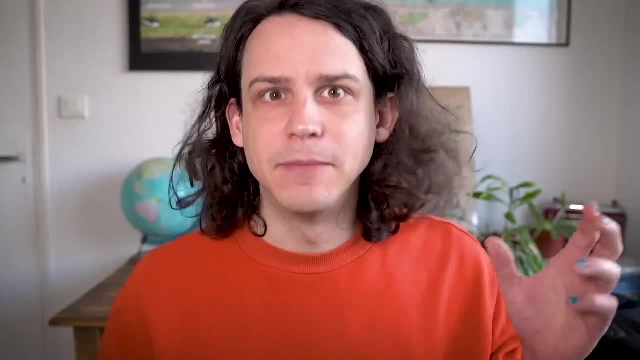 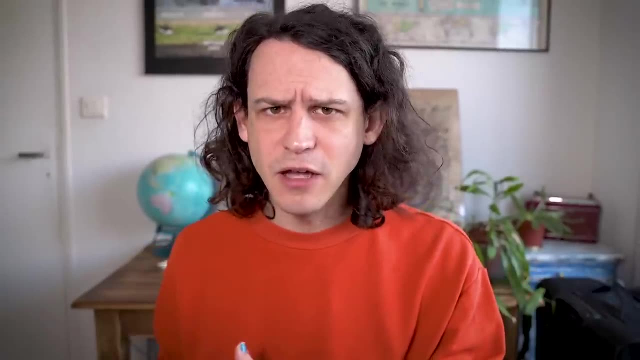 the replies from climate scientists. But maybe- and hear me out because this is going to sound crazy- but maybe the point isn't to ask questions and to learn, but maybe the point is to mislead What? No way, No way. 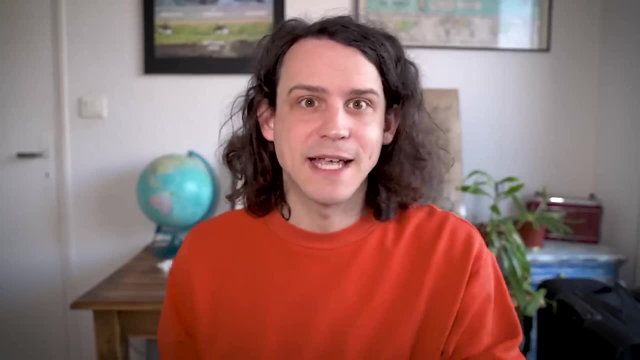 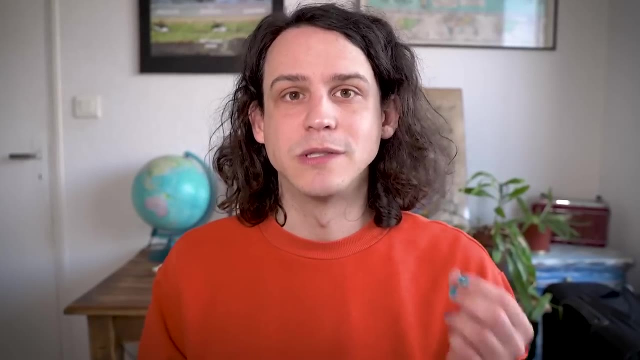 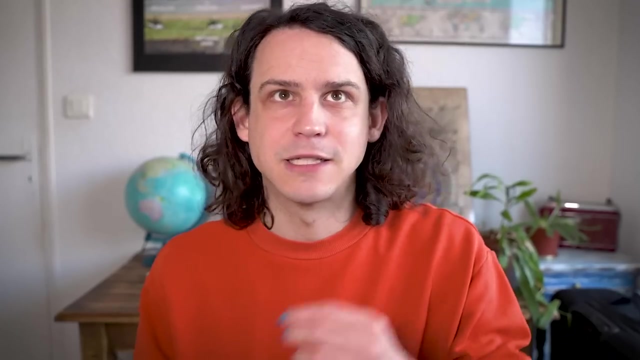 Because the thing is that if you actually care about the academic process and you actually care about the questions that you're posing, then you engage with the answers to those questions. But Jordan Peterson has a track record of doing the exact opposite, making statements that are misleading at best. 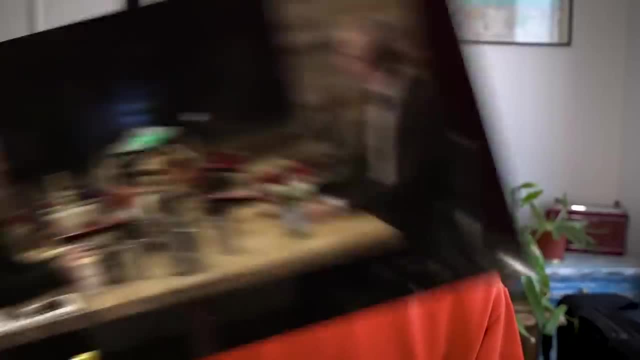 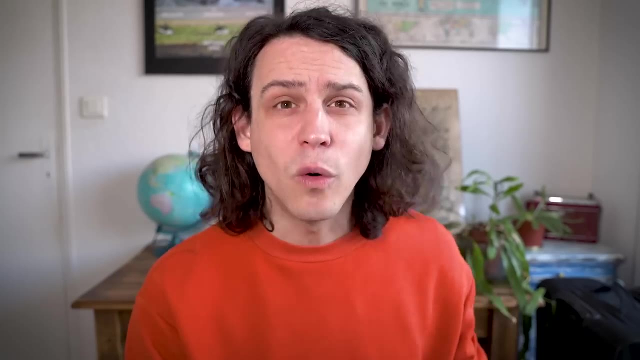 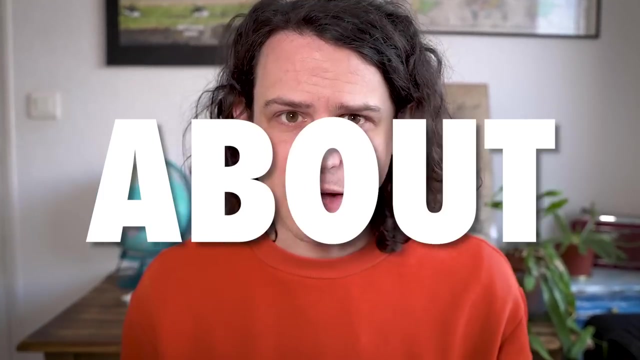 and straight up, making things up at worst. There's no such thing as climate right, Climate and everything are the same word. His scholarly tone makes this sound so thoughtful and sensible until you pause for one single second and you realise what are you talking about. 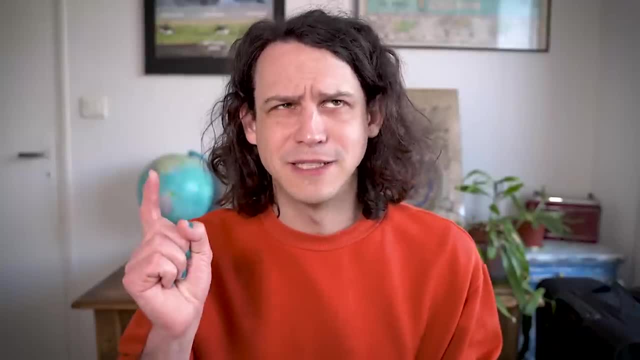 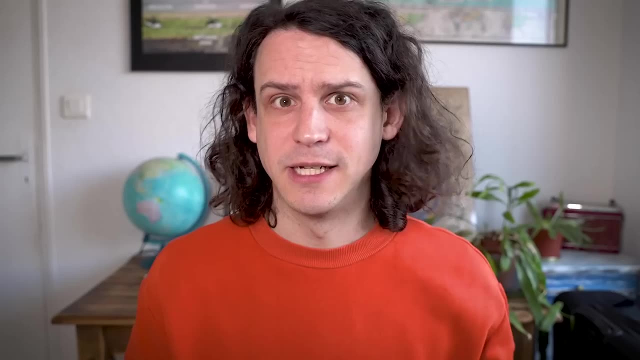 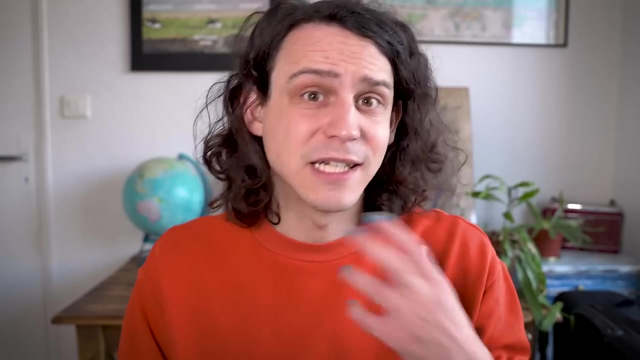 I don't have anything sensible to reply to this other than that climate definitely does exist and it definitely doesn't mean everything. But all this distraction is so key to climate change denial. Its entire purpose is to disrupt the science-based conversation and delay the action that the science is telling.